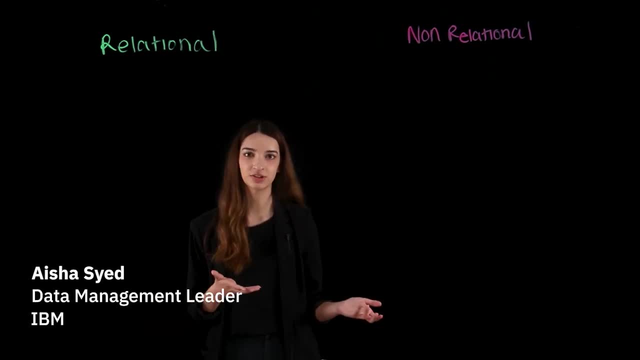 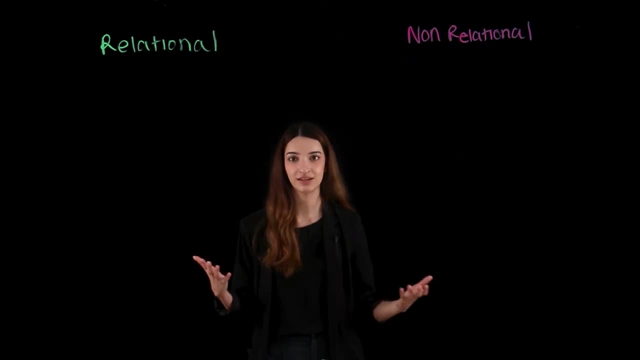 Hi everyone. today I'm going to be talking to you about relational versus non-relational databases. These are two different ways in which clients store the data that they have and operationalize it, And we know there is so much data that is coming into every single company today. 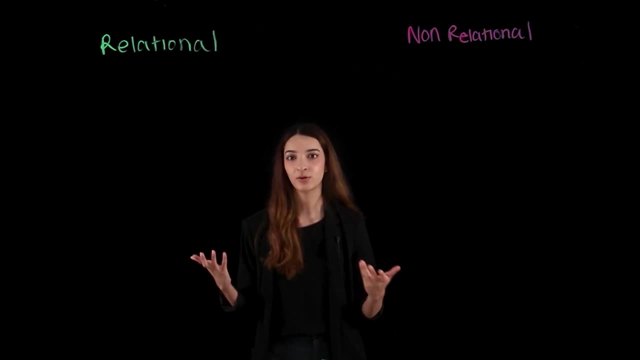 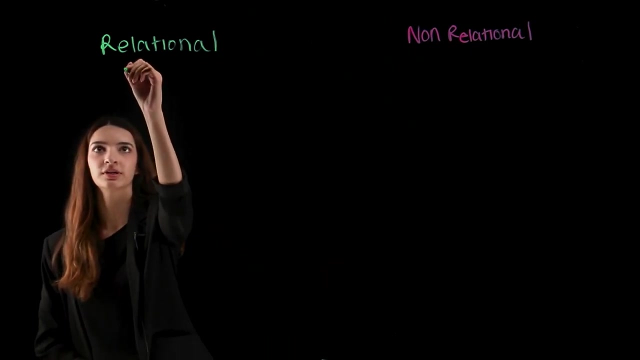 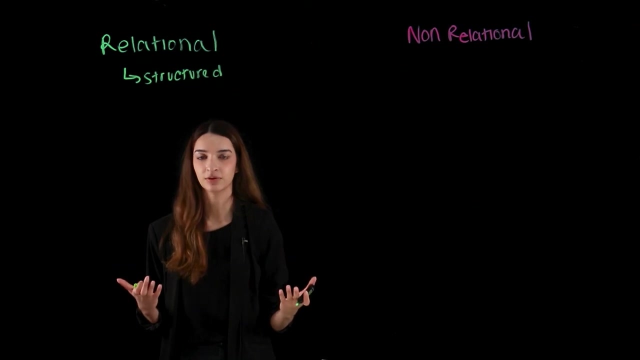 that it's important that customers have options for how they want to store that data. So let's start with relational databases. Relational databases are a very structured way to store your data. But to really understand a relational database, first we need to understand a table. 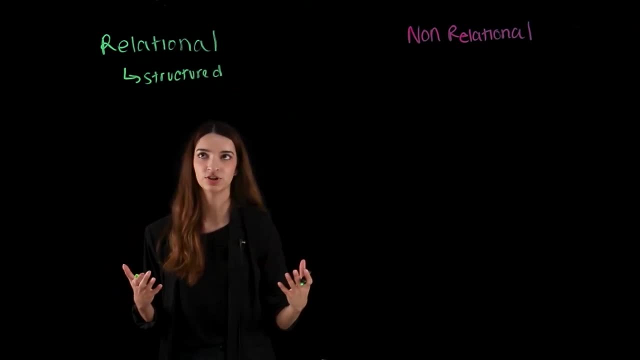 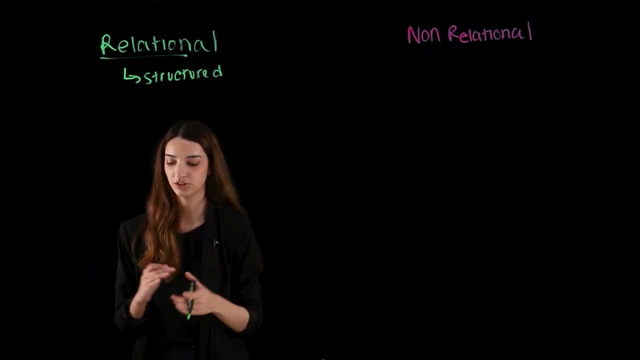 So all the data is stored in tables and those tables are connected to each other. That's why we have the name relational and we see relation in the name, because all these tables connect to each other. They all have relations with each other. So let's start with one table. 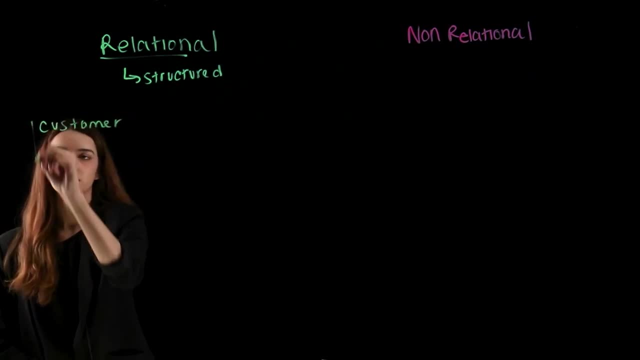 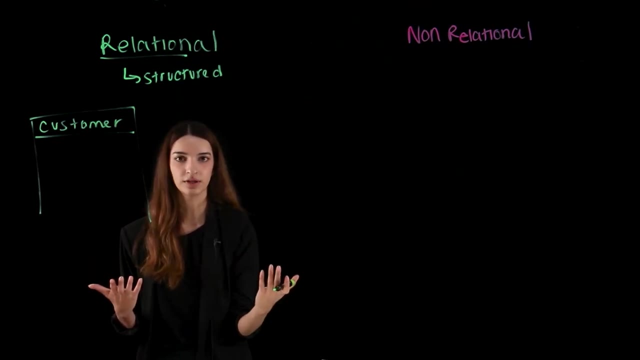 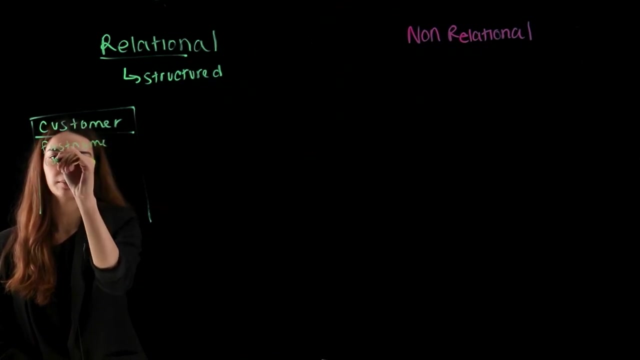 We have our customer, So each table revolves around a single entity, And with our customer, there is a lot of different information that we would want to know about them. right, We'd want to know what their first name is, their last name? 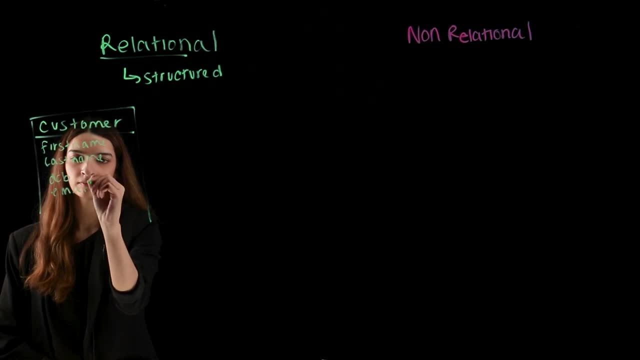 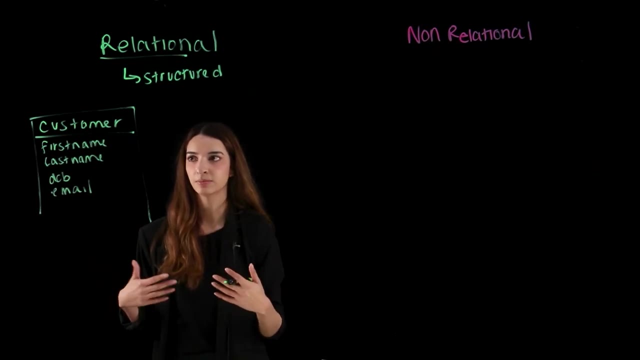 maybe their date of birth, their email and etc. etc. whatever other information would be relevant to know about the customer. But we might also have customers that have the same first name or the same last name and we need a way to uniquely identify each customer. 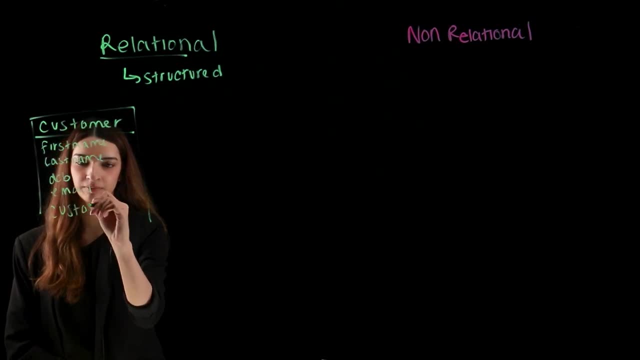 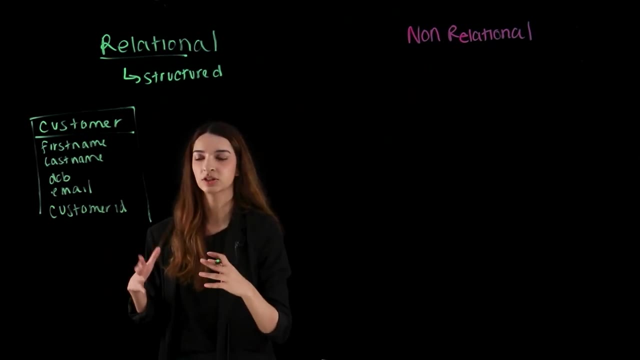 So that's why we have our primary key, which is our customer ID, And this is a unique identifier for each record in this table. But, like I said, with relational databases, we want to view each table as it connects to other tables. 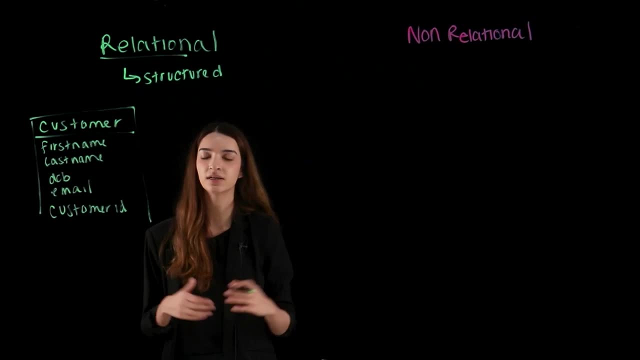 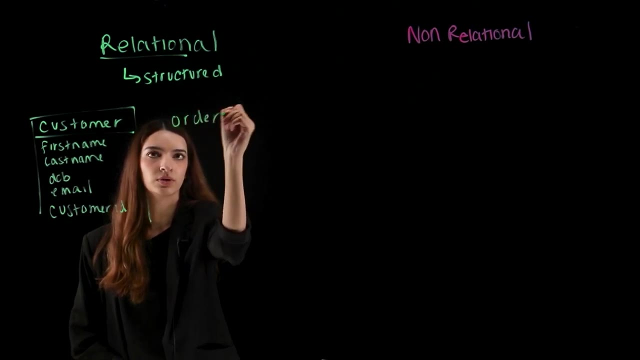 So let's think about what a customer does. A customer places an order, right? So an order is actually a separate entity that would connect to our customer table. So let's draw out our order table And what would we want to know about an order? 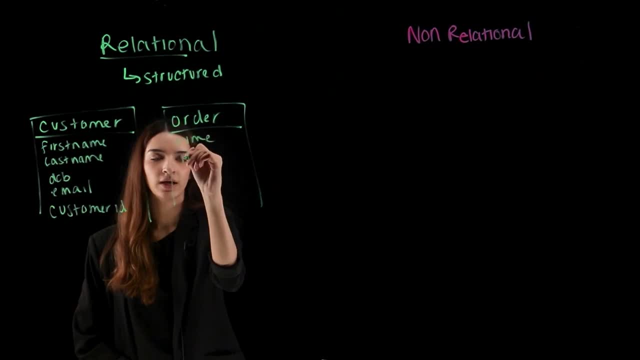 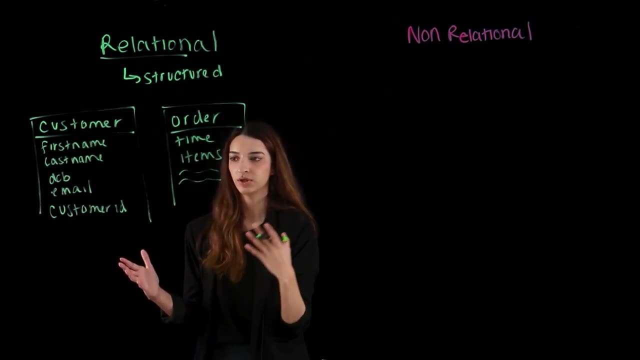 We'd want to know, maybe, what time it was placed, what items are in it and whatever else you think is relevant to the order. So that's what we need to know here, But again, like with the customer ID, we need a unique way to identify each order. 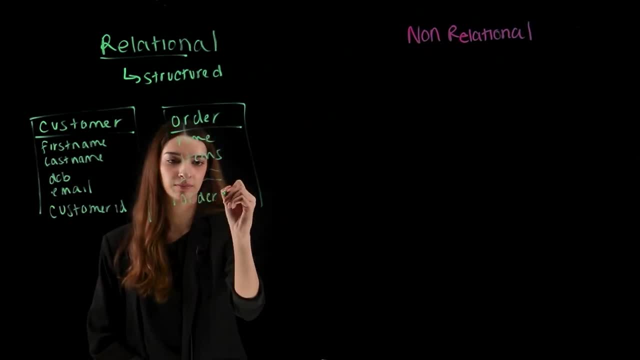 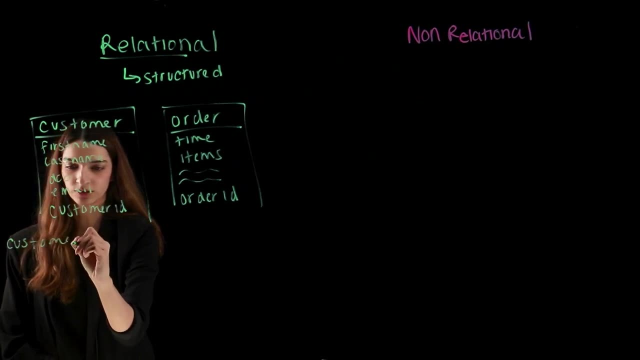 So we have another primary key here called an order ID, And if we look at each of these tables and we look at the data in them, we can really see how they connect to each other. So let's take a customer table, for example. 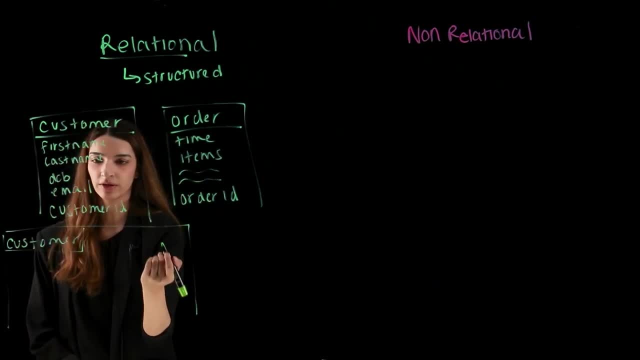 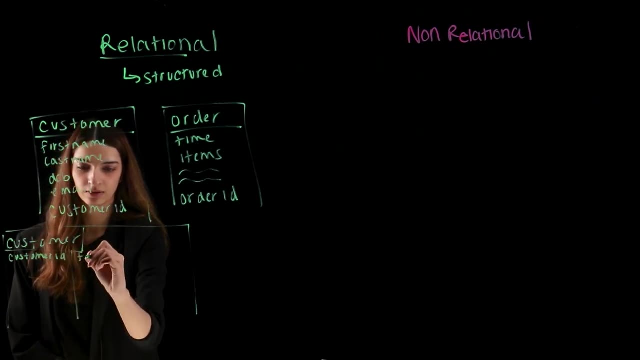 We know we have all these different pieces of information that are relevant to know about the customer. So I'm going to start with the customer ID And then we have their first name, last name, et cetera. So, like we said, each customer ID is unique. 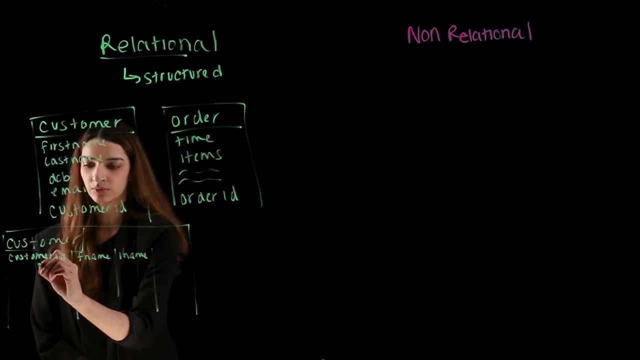 There's only one for each record in the database. So we have our first customer- Let's call him John Doe. Our second customer, let's say, is named Jane Smith, And third customer. we can change that. We can just continue populating information. 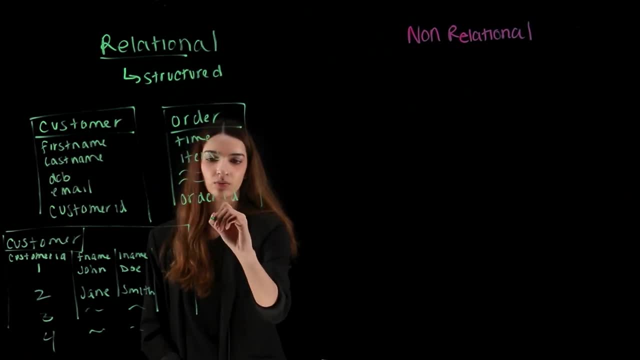 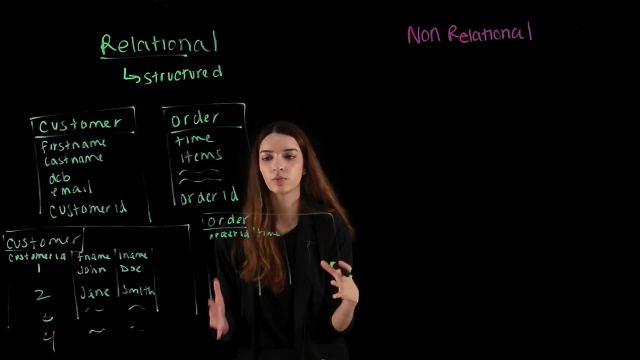 about every single customer that we have. And then with our order table, we start with our order ID And we have other information that we want to know: right Time items, et cetera. But what we also need to know is which customer placed what order right. 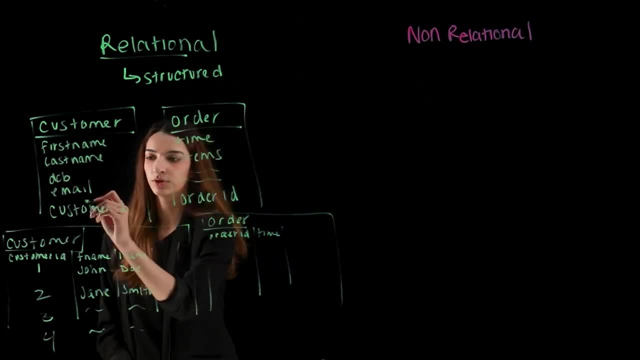 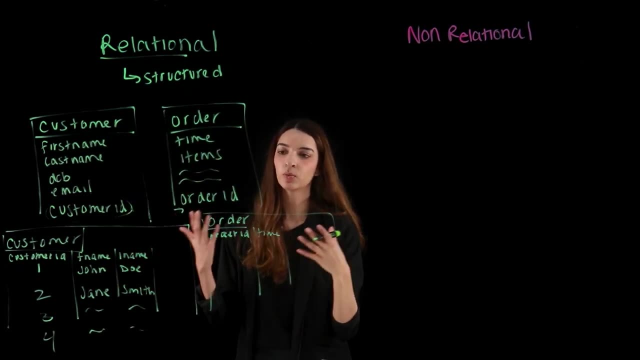 So in order to do that, we actually connect the customer ID to the order table, So we take this information and we move it over here. So in the customer table this is the primary key, But when we move it over, this becomes the foreign key. 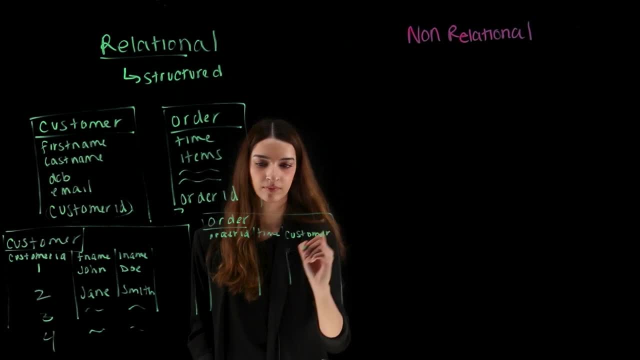 So now we can add in our customer ID here And we have our first order. It's placed at this time. Second order, third order, And looking at our customer ID, let's say that this is one And our second one is two. 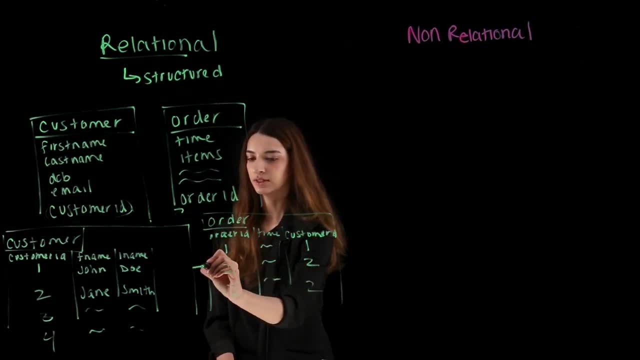 Our third one is also two And now we can see, through connecting these two databases, that customer, John Doe, made the first order- We see what time, what items. He also made the second order And Jane Smith made the third order. So, as we can see, with relational databases, 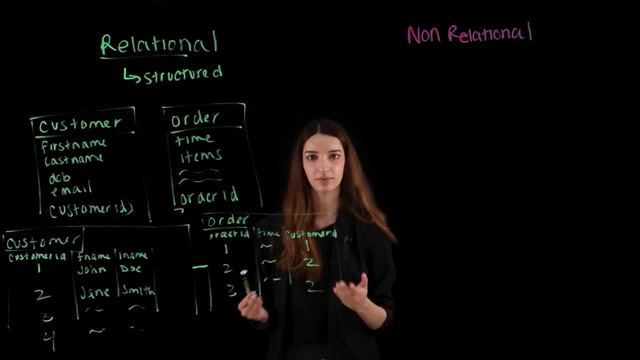 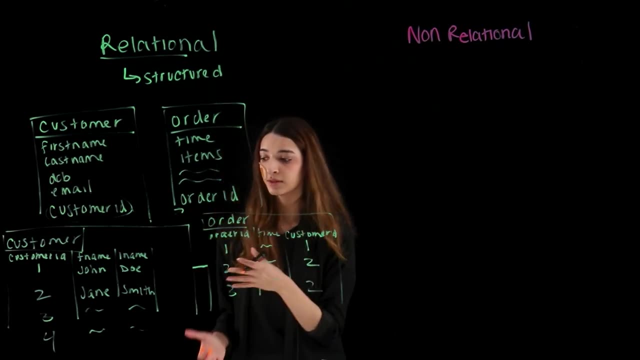 this is a very structured way to view the information that's coming into a company, But with that there's a lot of benefits that come in. So one of them is that the structure really ensures data consistency, And you can see that all the data that we have over here 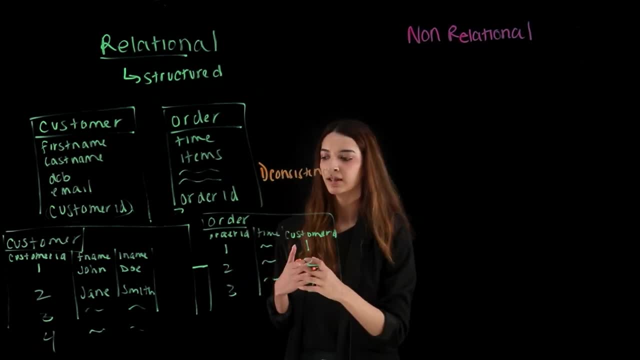 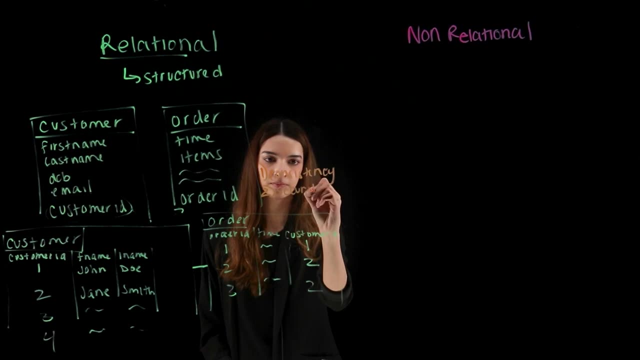 is very consistent, right? We can see that it's easy to manage that data and easy to get an overview of what is in your database. This also helps with security. So let's say that you are a hospital and you have a lot of patients. 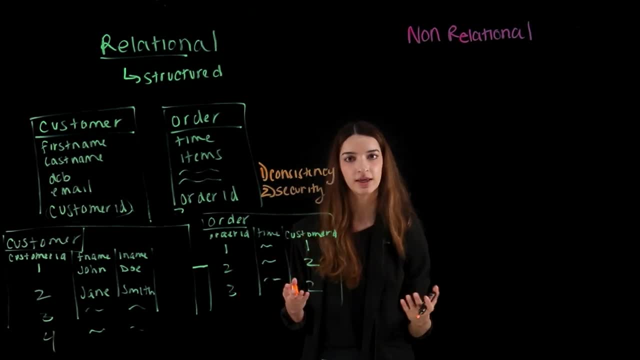 You have information about their medical history, what medications they're taking. That is all protected information. So, through using a relational database, you can encrypt certain tables, you can hide information and you can make sure the right people have access to the right data. 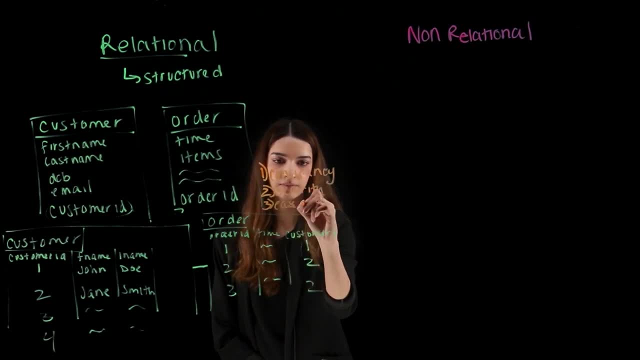 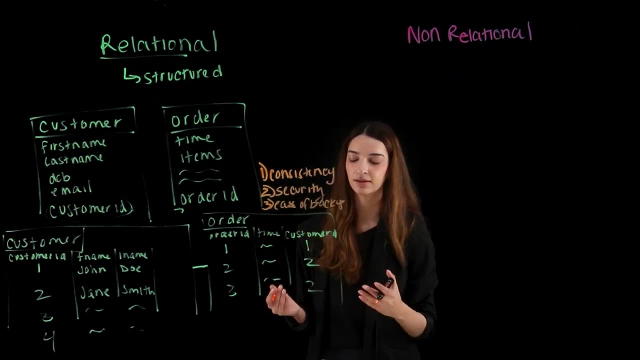 And then, finally, we have ease of backup and recovery. So, because this data is very consistent and at all times it remains consistent, it's easy to save the database at any point and easily recover it from what you recently had. So this gives us an idea of what a relational database looks like. 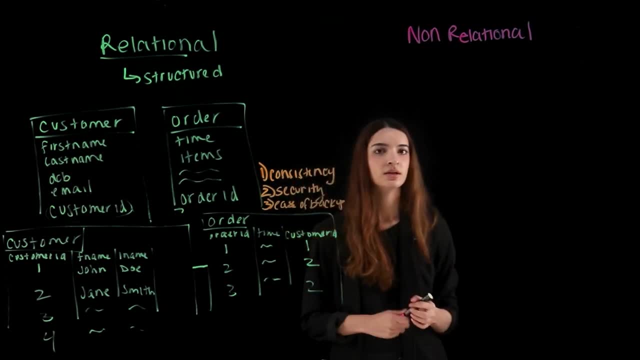 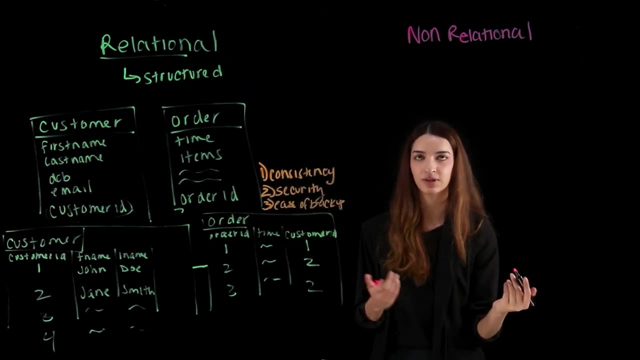 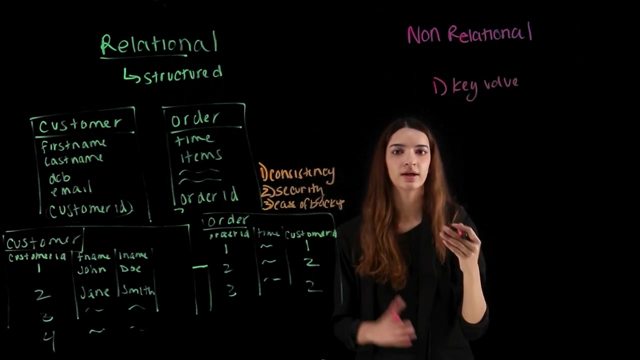 Now, on the other hand, we have non-relational databases, So this is a break from the very structured approach of a relational database. There are a few different types of non-relational databases. First, we have key value databases, And this shows data as a key and a value right. 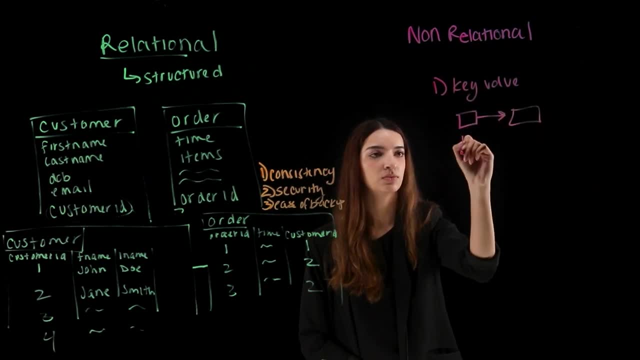 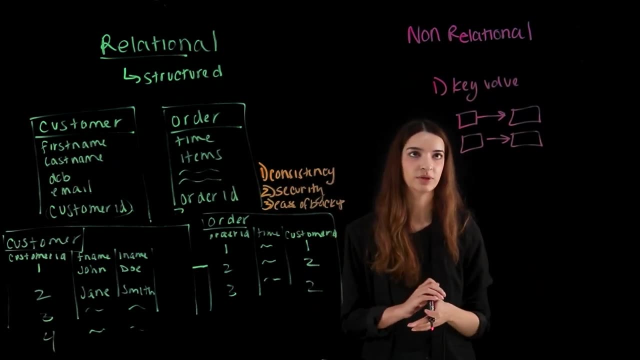 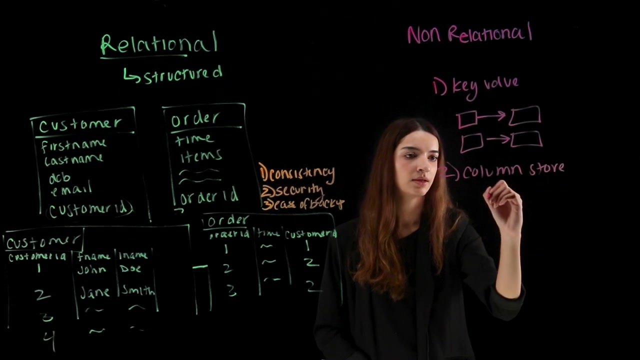 We have one key that ties to one unique value, another key that ties to another unique value, and you can retrieve these values through plugging in the keys and getting that information back. We also have column store databases And this stores data in separate columns. 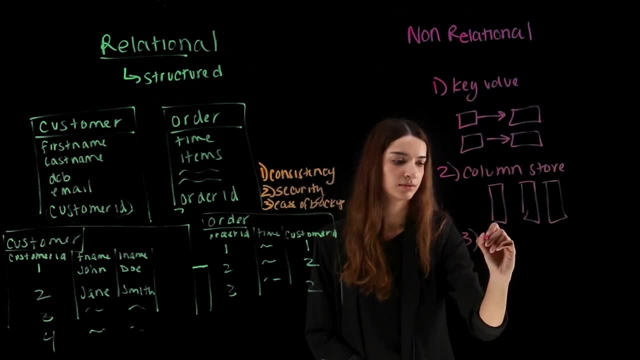 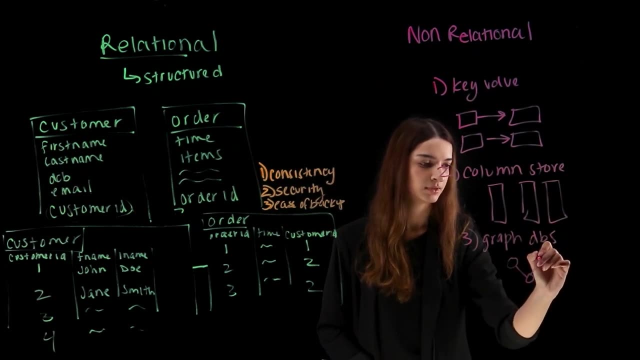 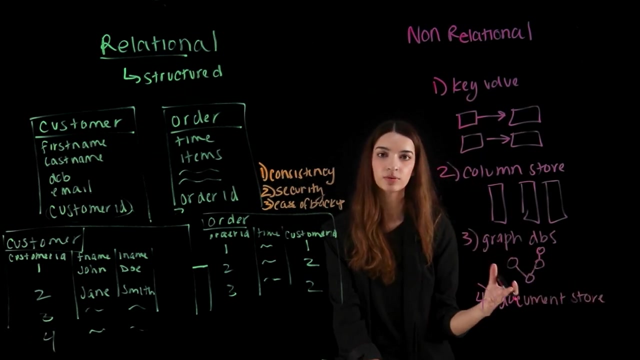 and is optimized for performance. And then we have graph databases, So this shows different entities in the database and how they connect to each other in a graphical way. And finally, we have our document store databases, So this has data in documents. 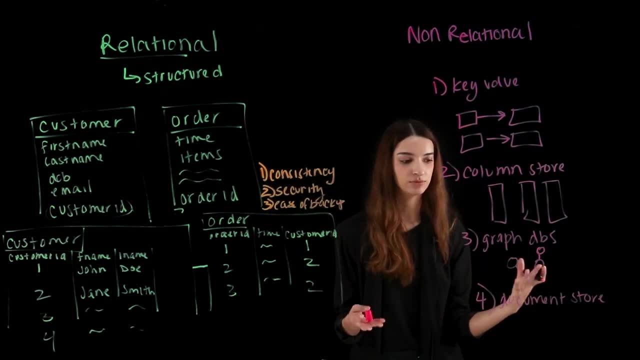 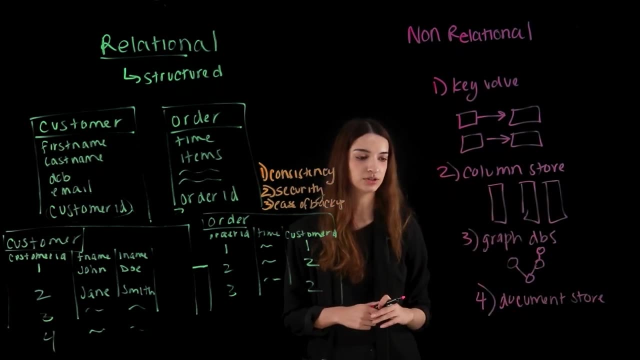 and a group of documents is called a collection And you can essentially retrieve the information that relates to a single collection. So you see that there are a lot more options here with the non-relational databases, And that's really why customers might choose a non-relational option. 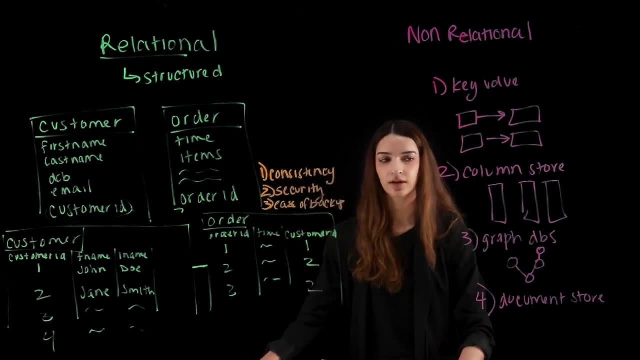 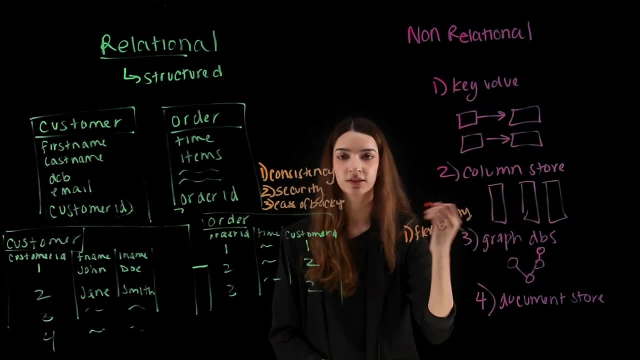 as opposed to a relational one. There is added flexibility in going with a non-relational database. So that's really one of the key differentiators and why customers choose non-relational over relational. It also has high scalability. It's easy to scale non-relational databases out horizontally.